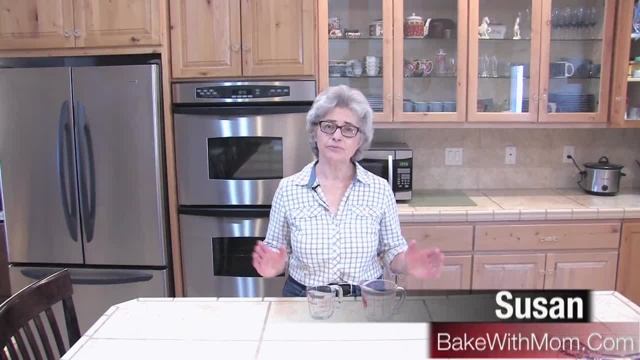 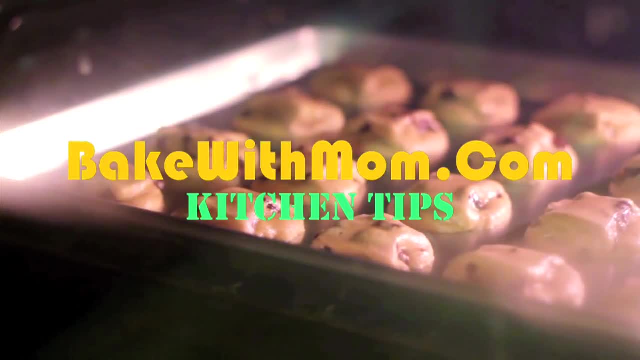 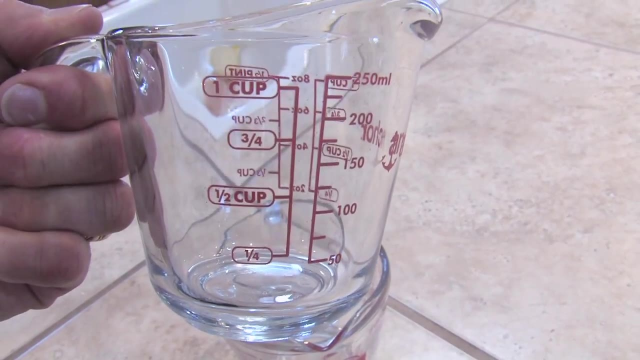 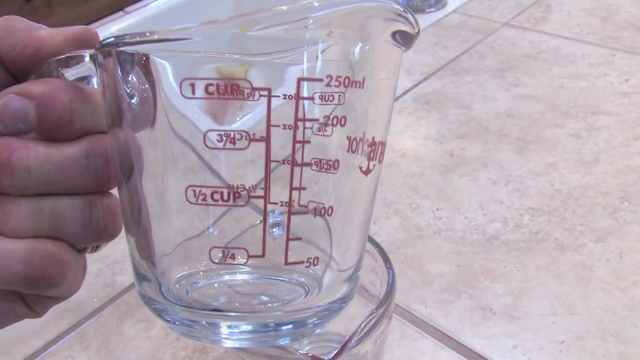 Hi, I'm Susan from bakewithmomcom. Today I am going to tell you how to properly use a measuring cup. So your cups normally are marked and the one quarter cup is obviously the one on the very bottom, and then it's a half cup, three quarters of a cup and one cup If you have a two cup measure. 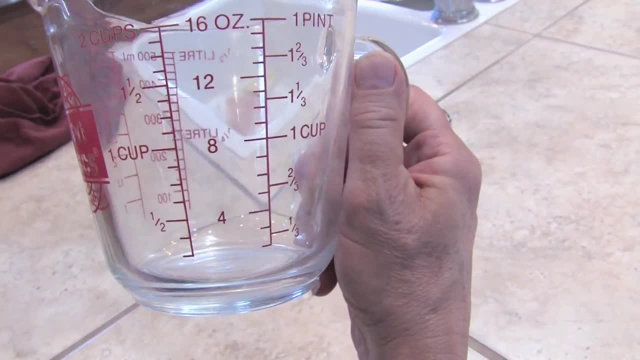 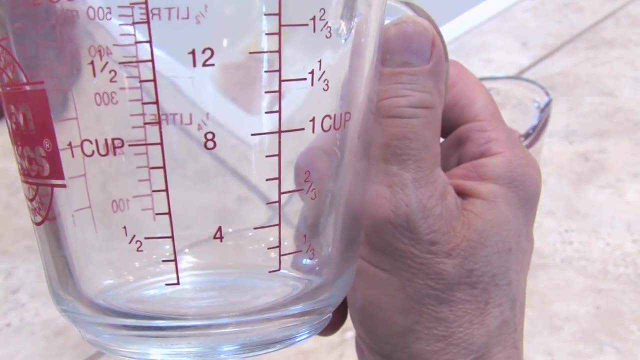 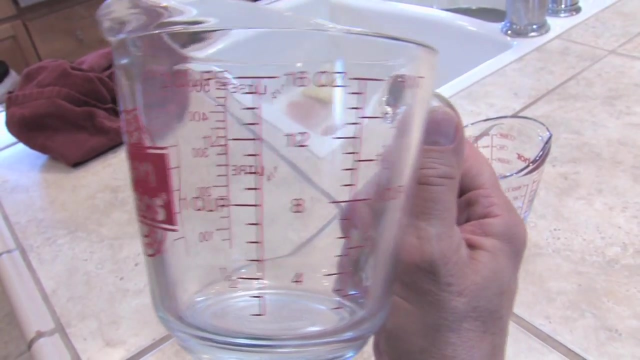 you won't have all of them marked, but the line at the very bottom would be a quarter of a cup, and a half a cup is marked. then three quarters of a cup would be halfway between a half a cup and a cup, and then your one cup. I had watched a show where a lady was supposed to use a quarter. 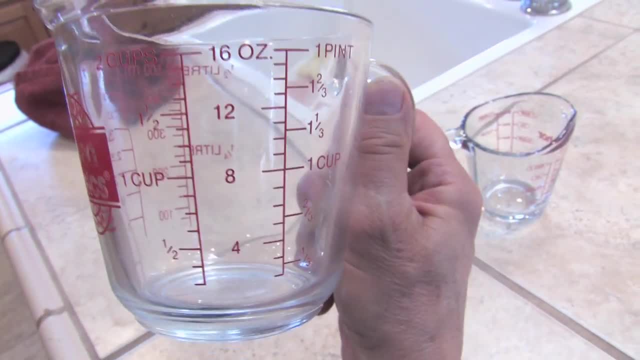 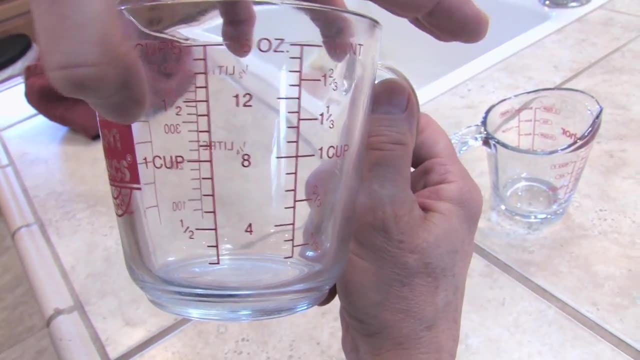 of a cup of oil and what she did is she did way up here- she did a cup and a quarter, because she saw a quarter cup marked just below the other cup to mark, and that's what she did. So wouldn't you notice my line at the very bottom would be a quarter of a cup and a half a cup is marked Then. 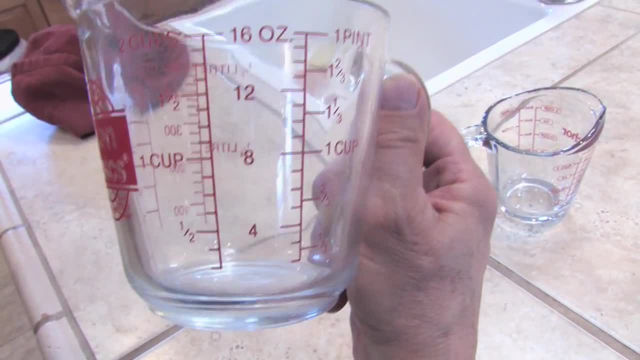 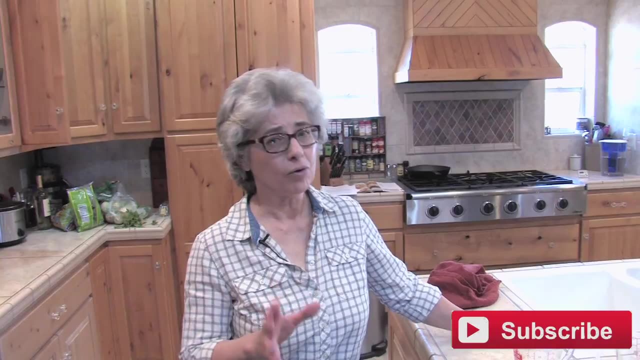 quarter mark on the, the cup that she was using, instead of going down here. That ruined her recipe because she used far too much oil for her recipe- A whole cup extra. So I hope this helps you out. If you need any more tips, check my site at. bakewithmomcom and subscribe. 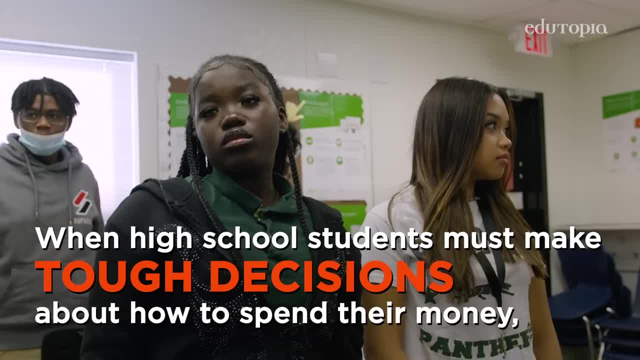 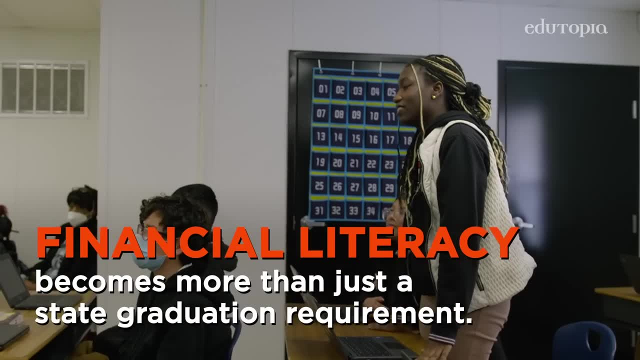 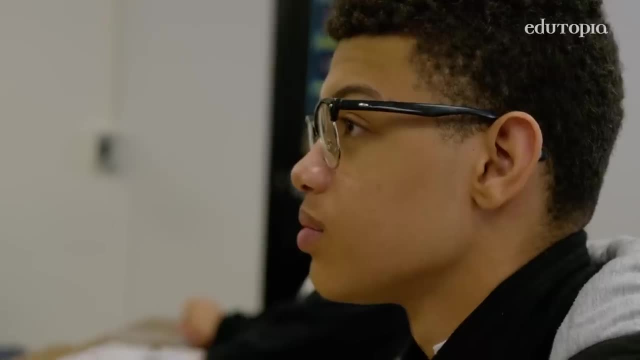 Would you rather drive to work if it cost you $150 per month to park, or would you rather catch the metro and it's only going to cost you $25?? I'm going to take the metro. While students may not need to know an algebraic expression to get through life's events, they